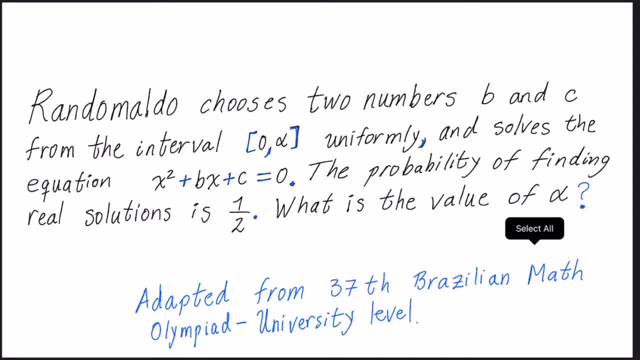 Hello everyone. today we will solve an interesting problem that mixes algebra and probability, and some parts of integral calculus too. So what is the problem? The problem is like we have like random model. this is our character. choose two numbers, b and c, from the interval from 0 to alpha. 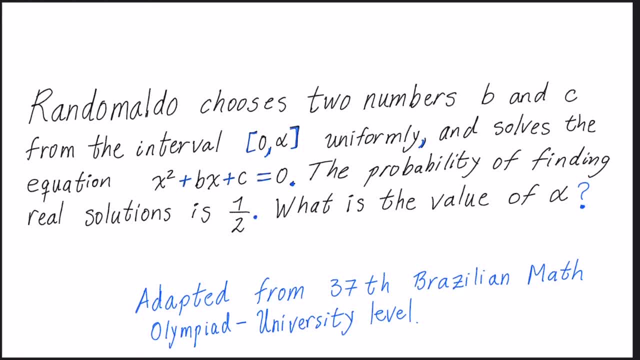 uniformly. Also, we have to consider here the fact that the numbers b and c are taken from 0 to alpha independently And solves the equation x squared plus bx plus c, equal to 0. The probability of finding real solutions is 1 divided 2.. What is the value of alpha in this case? So this is a problem. 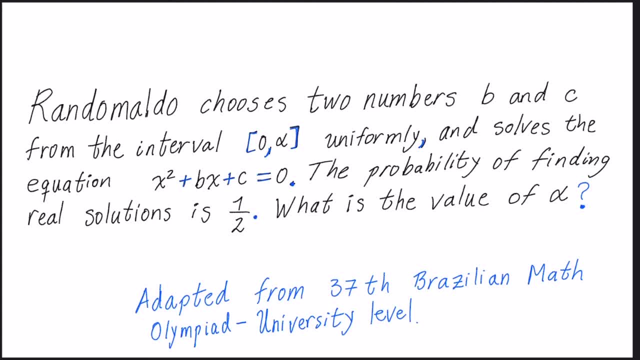 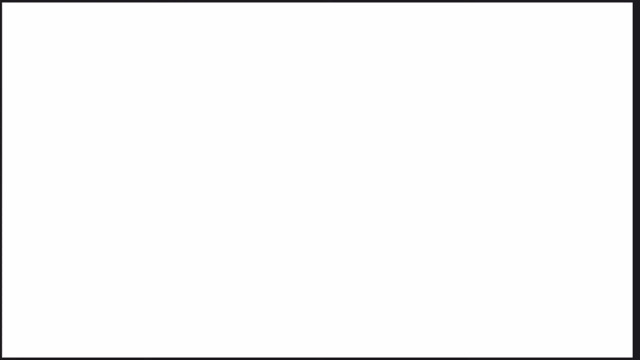 adopted from the 37th Brazilian Math Olympiad. in the case where the answer is not the answer, in that case we will find the answer of the problem. In this case, the problem is just 1 divided by 2, the university level. so how we can start this problem. so we have at first the 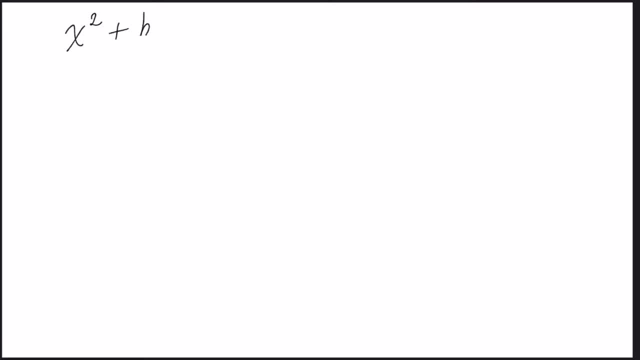 question of the form: x squared plus B, X plus C equal to 0. so we know that this problem has real solutions with a probability of 1 divided 2. so which condition can be transformed to make this equation to have real solutions? so we know from algebra that if B square minus 4 by 1, by C, is bigger or equal. 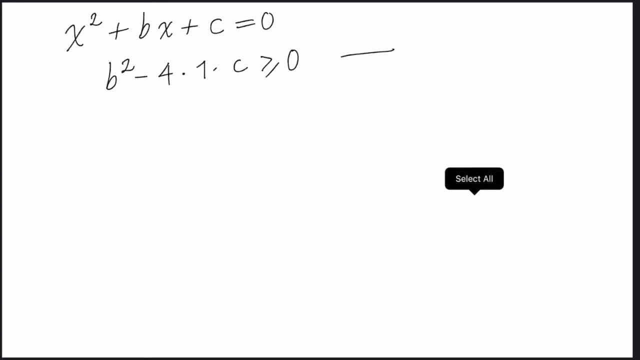 than 0, then we have real solutions, okay. so we use this hypothesis from here. we know this, it's okay. and also so we can rewrite this like B square is bigger or equal than C, but 4 multiplied by C. okay, now we know that B and C are taking both of them from a uniform. 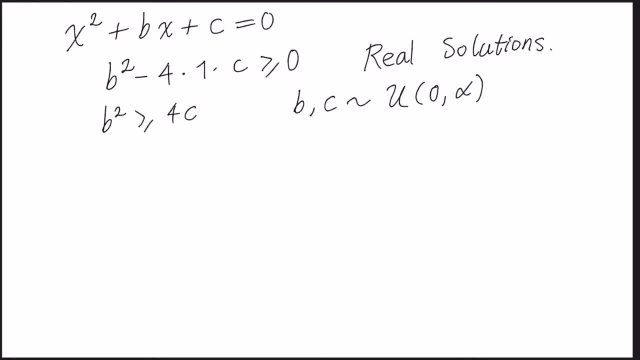 distribution which has values from zero to alpha. that is really important to note. that B and C are independent, okay. so what does it mean? it means that we can create a Cartesian and we can write B and C as the labels of the axis and we can write B and C as the labels of the axis. we can write B and C as the labels of the axis. 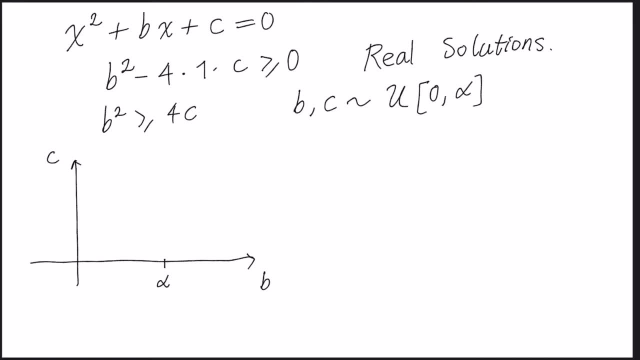 Also, we can write for B from 0 to alpha and for C from 0 to alpha2.. Okay, so why can we do this? Because B and C are independent, so they can be seen as values in orthogonal axes And we can complete the space that they will take as an square with side alpha. 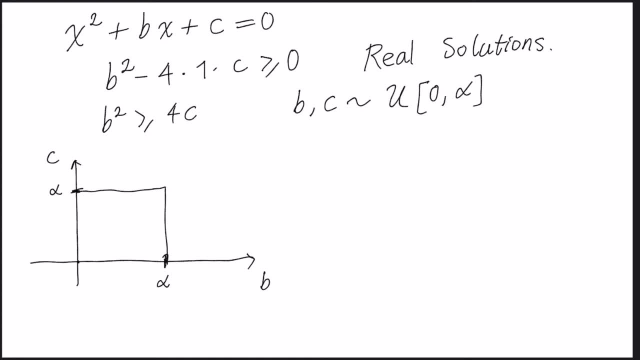 Okay. so now we have to draw this inequality. So let me rewrite here properly: So B squared divided, B squared divided by 4 is bigger or equal than C. Okay, so remember, if we want to obtain the graph of one inequality, then we have to graph the quality. 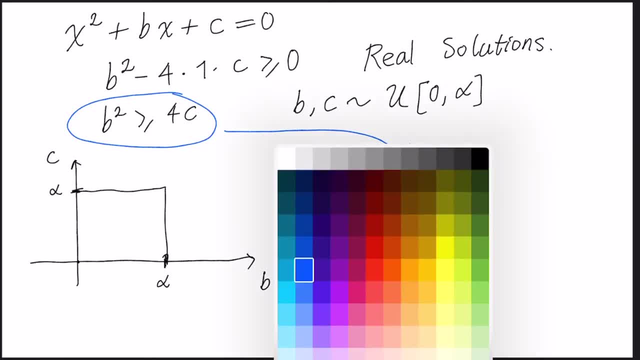 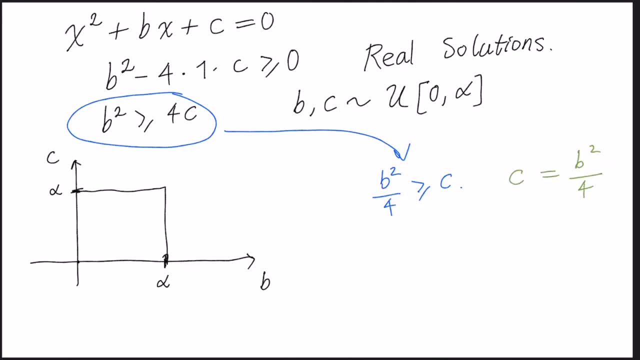 So we will work with the equality given by C equal to B squared divided by 4.. Okay, so we have two options. We know very well. So this is a parabola. it is well-known fact. this is a parabola and there are two options. 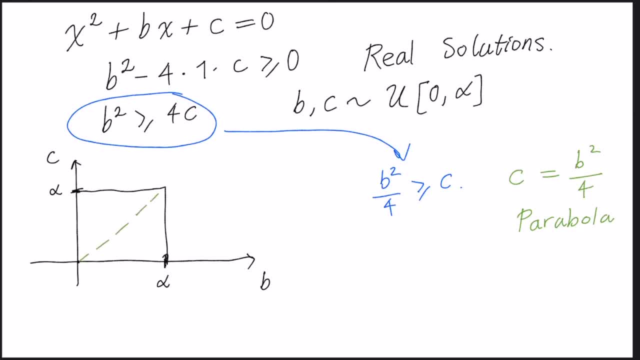 What are the options? So here I will just put in the dotted line this is G equal to X, I equal to X, and we have two options. The first option is the following: The first option is that the curve follows this path. 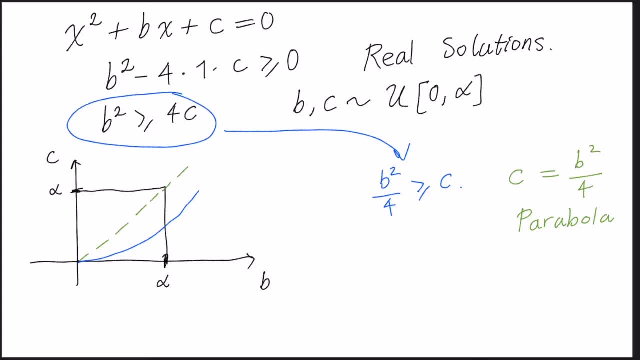 And where is the problem here? The problem here is that we know that the probability of Probability- Oh sorry, Probability- of B squared bigger or equal than 4C is equal to 1 divided 2.. It means that we will divide the square in two parts that have equal area. 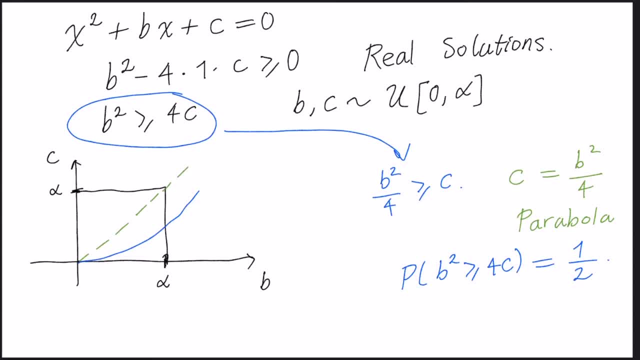 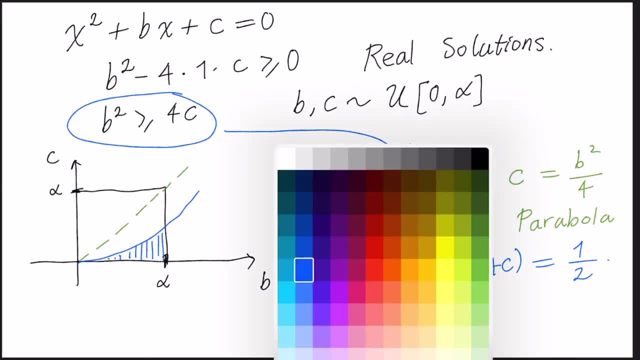 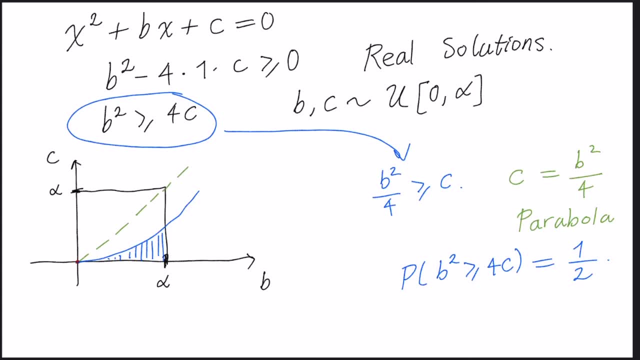 not a good option. so what is the other possibility? the other possibility that I will show in red, as you can see, is that the cure has this shape: yes, so this is more possible because it can: is below g equal to x, y equal to x and also can. 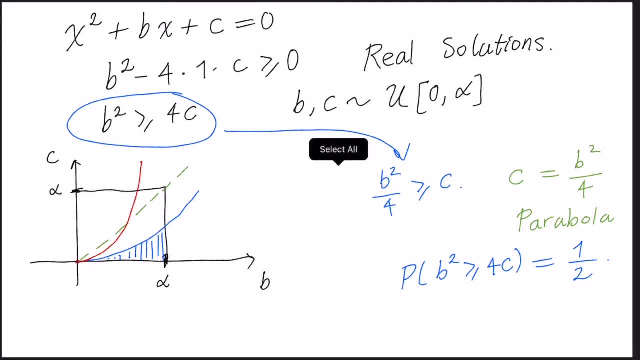 overcome y equal to x, so it's possible that this area is equal to x to this area. of course, this is it doesn't seem to be possible from my figure, but we will find conditions for alpha such that it will be true. okay, so I will remove the area shaded and I will now shade the area that we require to. 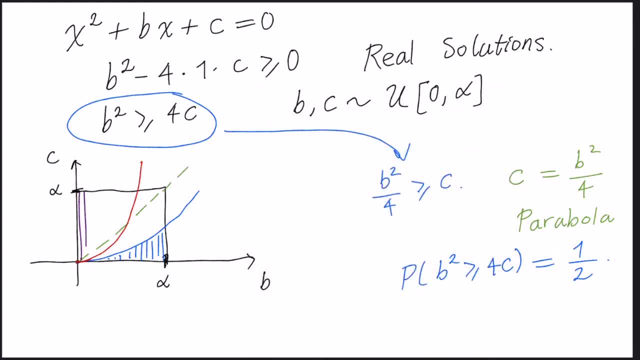 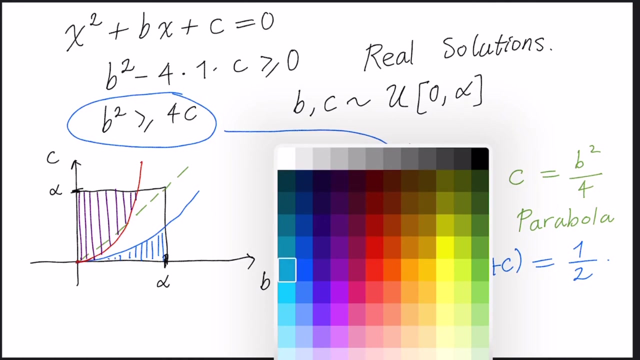 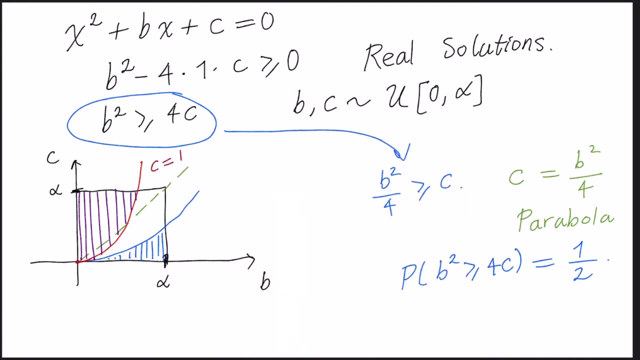 find using purple. so we require to find this area. yes, so how can we obtain the area? the area is just an integral, as it can be seen, and the red, the red curve, can be written as C equal to B square divided 4. so I will note this with the letter A, so A is 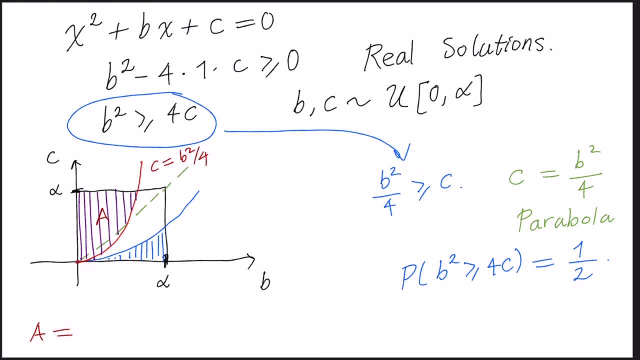 equal to integral from. okay, what is the area here if we see it as a vertical, vertical, vertical, vertical, vertical, integral? I will try to make a double integral here. it's a little bit problem, why? because we have to know where. what is this point? it's not difficult to know it. 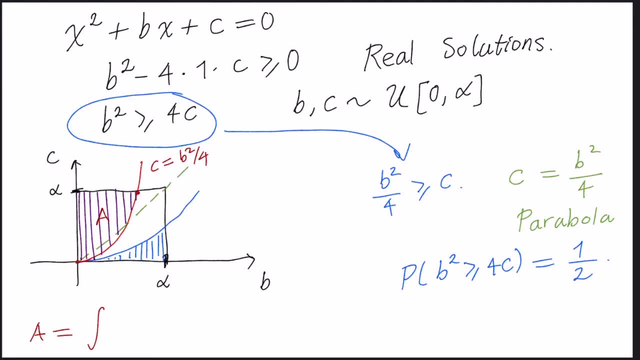 but it takes time. but if we change our point of view and instead of supposing that the integral is vertical domain and instead of that we put an horizontal domain and instead of that we put an horizontal, Then it will be more simple to obtain the answer. Why? Because the integral will go from 0 to alpha, Yes, And also it will go from 0 to. in this case, we have to obtain b in terms of c. 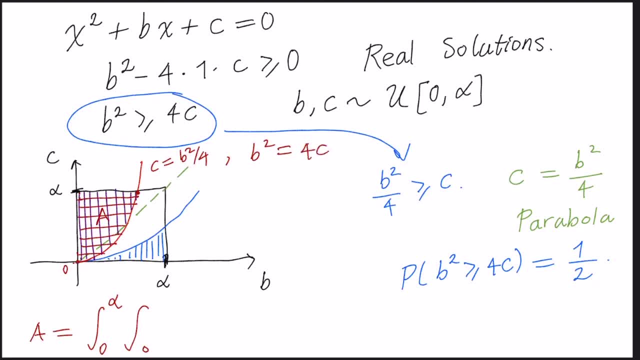 So b squared is equal to 4 by c. So b is equal to root square, or 4 by c, or the same that 2 root square of c. Okay, So even I don't need to make a double integral, I can do it. We don't normal integral of calculus. 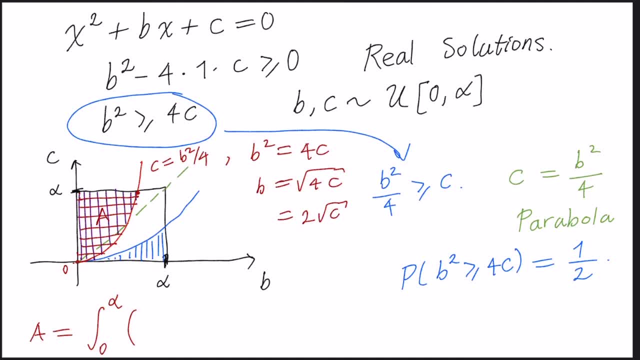 So the most right part to root square of c Minus the left part- Remember we have this- This is 0. And in this case we will put by the c: Okay, This is just a common integral, Can be solved easily. 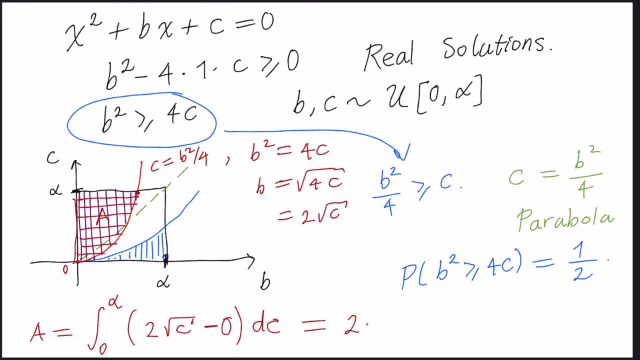 So it's equal to 2 by 2 divided 3 by c, 3 divided 2, from 0 to alpha, Or this is the same that 4 divided 3 by alpha, 3 divided 2.. Okay, So what is the next step here? So we know. the area is 4 divided 3, multiplied by alpha, 3 divided 2.. 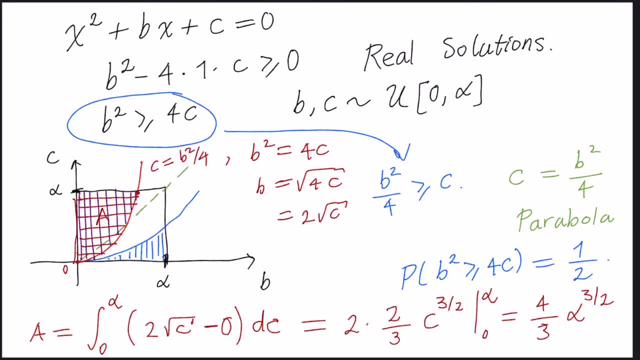 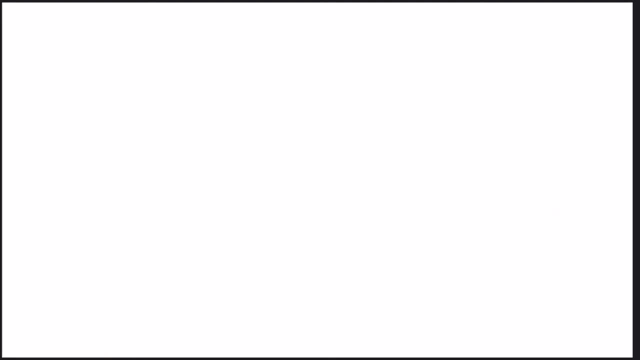 And we have to remember that for a uniform distribution The probability is just equal to the same than Laplacian approach. We will say: just like the probability in this case, 1 divided 2, is equal to, The probability that we found was 4 divided 3 by alpha, 3 divided 2 divided by the total area of the square. 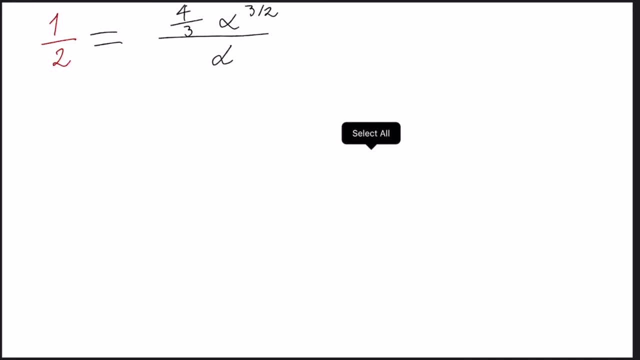 This is Alpha by alpha. But why? Because, remember, it's a square, And it's square with side alpha. So what? just the area is the multiplication of the sides. So 4 divided 3.. Multiply by alpha: 3 divided 2.. 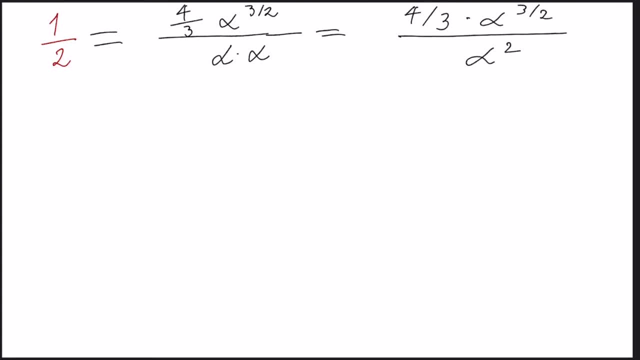 Divided alpha square. Okay, So we have finally 1 divided 2. It's equal to 4 divided 3.. Here we make some algebra: 2.. So on the denominator 2 minus 3 divided 2.. And now we just arrange little bit. 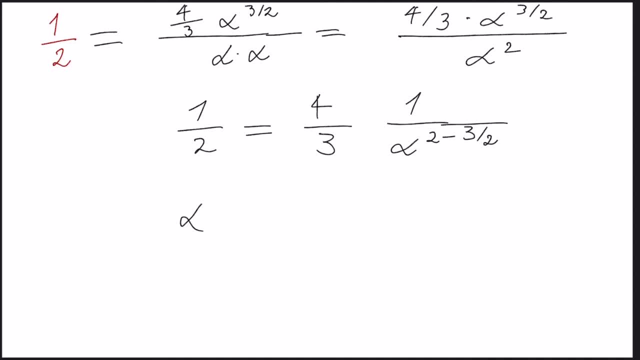 So we have alpha at 1 divided 2. Is equal to 8.. 8 divided 3.. Finally, We just make Square to both sides And we will obtain that alpha. Remember alpha was a positive number, So it's okay. 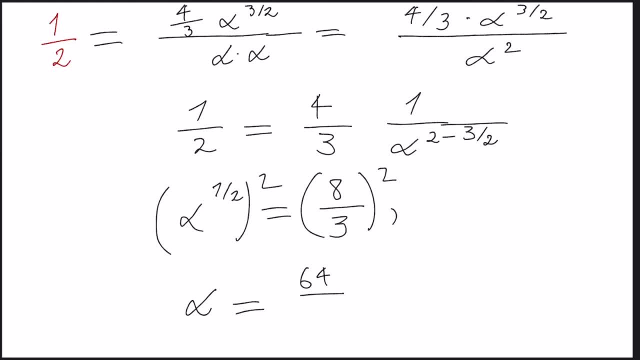 Is equal to 64 divided 9.. And This is the value That makes us to obtain Real solutions with a probability equal to 1 divided 2.. So that is all for today. I hope you have enjoyed this video. Also, remember that additional or alternative solutions are welcome. Thank you so much. Have a good day to everybody.